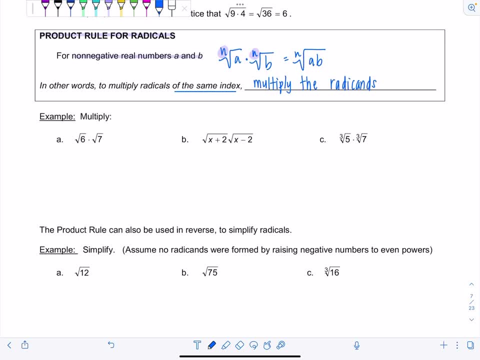 So, example a: we're going to multiply square root of 6 times square root of 7.. So all you're going to do, they're both the same index. right Square root, the index is 2, n is 2. And I'm going to put underneath the radicals 6. 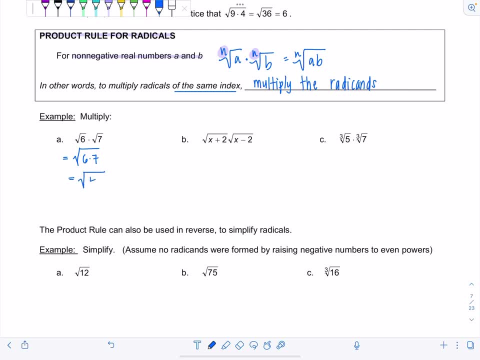 times 7.. And then this will simplify square root of 42.. That's it All right. good Example b: x plus 2 times x minus 2.. I can put each of those terms underneath the radical. That's a difference of. 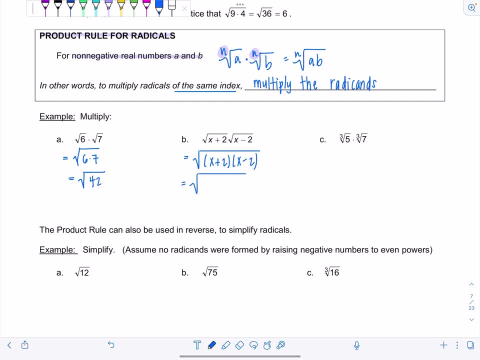 two squares when I multiply it out right, Since we have conjugate pairs. So this is going to be rad x squared minus 4 under the radical. Does it simplify further? Can I write something like x minus 2?? No way, don't even think about it. As we talked about in the last video, 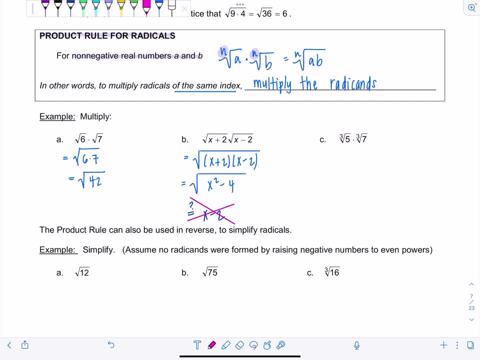 you cannot split up a radical over addition or subtraction. Okay, so leave it alone. Let's just box it To keep you from doing something bizarre. Let's box our final answers, It'll keep us honest. Okay, very nice. Example c: oh, cube roots, Cube root of 5 times cube root of 7.. So you're just 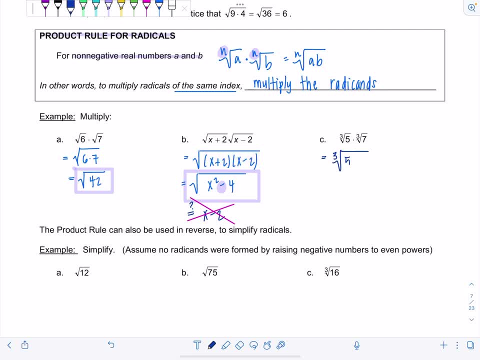 going to multiply 5 times 7 and put them underneath the same radical together. Make sure you write the index 3, okay, Don't be so quick that you forget, because otherwise it means something else. It means square root. So this is cube root of 35.. Beautiful. 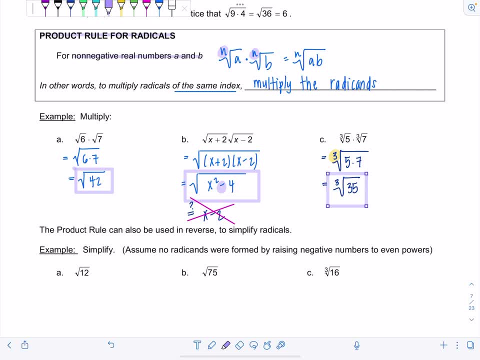 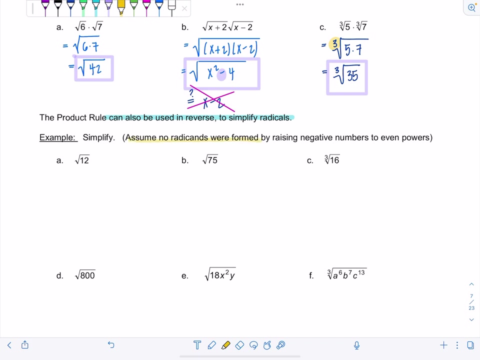 Now the product rule can also be used in reverse, And we can use it in reverse to simplify radicals. Okay, I'm going to show you how. right now The example tells us: simplify. And then here's a nice little disclaimer that we first brought up in the last video: Assume no radicands. 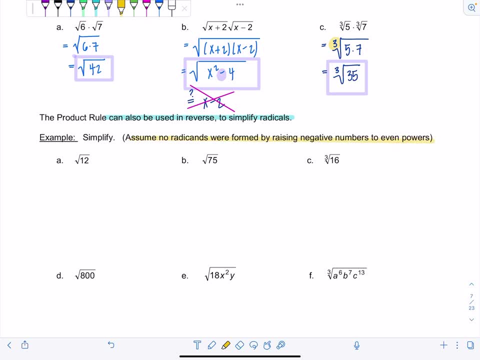 were formed by raising negative numbers to even powers. What that means is you don't need to worry about putting absolute value when simplifying, because they told us none of the variables represent negative quantities. But remember we learned last lesson that if they don't put this, 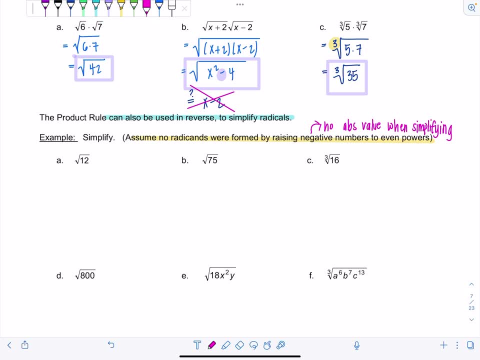 little disclaimer, then you do need to proceed with more caution, okay, All right, so here we're going to simplify, And the idea is: you want to factor the radicand- okay, in such a way that it's broken up into a product of the largest perfect square that goes into it. 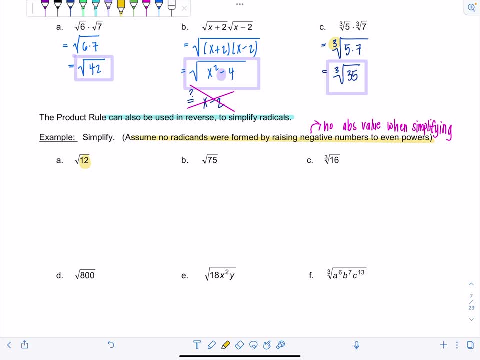 and then some other number. What do I mean? Well, 12 factors in a variety of ways. It's like, for example, 12 factors into 6 times 2, okay, But that would not be helpful to write it as such. 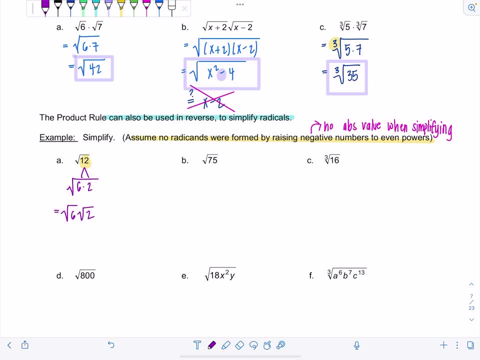 because then it would simplify square root of 6, square root of 2.. And who cares? Neither 6 nor 2 are perfect squares, So that's not going to be useful. A better way to factor 12 is to break it. 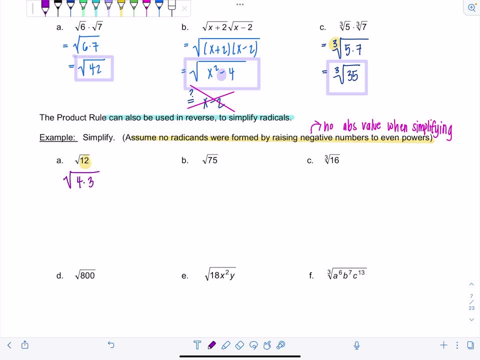 up as square root of 4 times 3.. Then I can split the radical now square root of 4, square root of 3. And notice, 4 is a perfect square. so this simplifies into 2 rad 3,. okay, So it is key. 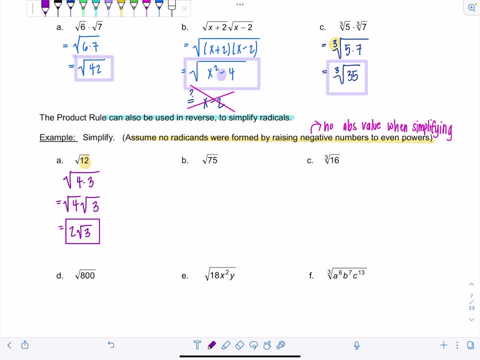 that you do know your perfect squares very well. Some people are all about these little factor trees when they simplify radicals because that's how their teachers showed them prior. If it's working for you, you live your life. You simplify the way you do. I don't like factor trees and I think this is a cleaner. It's a little bit more. 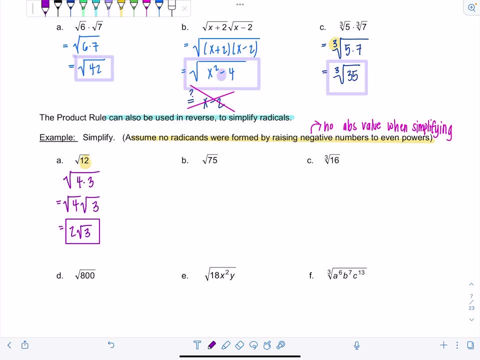 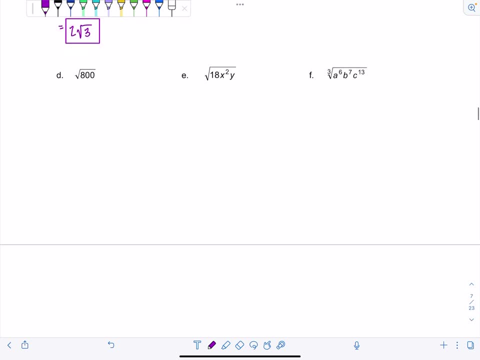 advanced, but you can handle it. You're not watching this channel, I think for kicks, Okay. so example B, square root of 75.. I thought it would be a good idea. Let's make a little list of all the perfect squares in case you're not familiar. 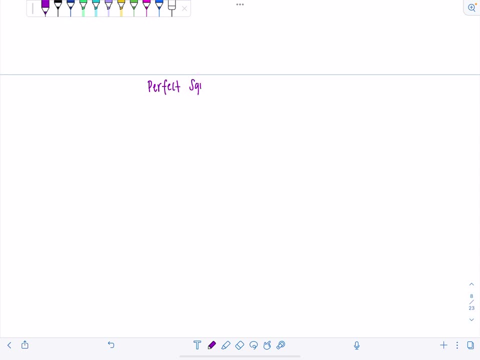 And then you can have them for reference. okay, Perfect squares. So 1 squared 1.. 2 squared 4.. 3 squared 9.. 4 squared 16.. 5 squared 25.. Oops, my brain was. 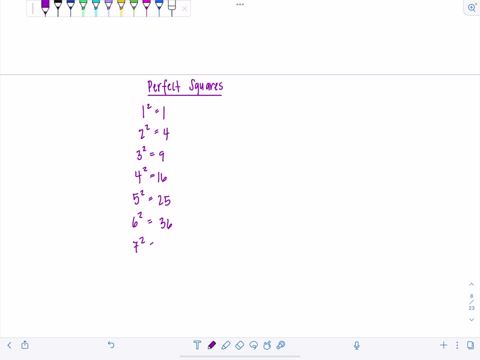 going to the next one: 6 squared 36.. 7 squared 49.. 8 squared 64.. 9 squared 81.. 10 squared 100.. 11,, 121.. 12,, 144.. 13,, 169.. 14.. I want to say 196.. Give me one second. 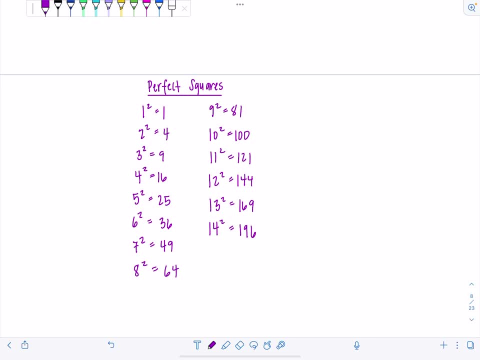 Yes, 196,. 15 squared 225.. Shall we keep going? I don't know. 16 squared 256.. 17 squared- This one's 289.. Yes, 18 squared 324.. These won't come up often. 19 squared. 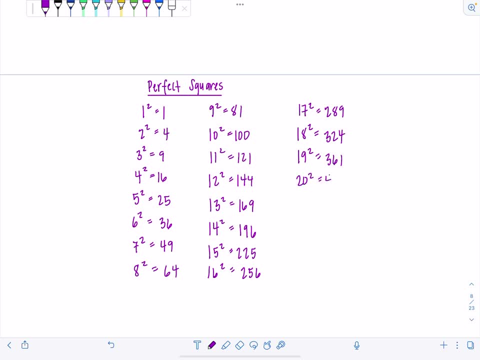 361.. And then 20 squared is 400.. Okay, I'd say, as long as you know, up to about like 12 squared, you're in good shape, okay. So the idea is, you want to find which perfect square, the largest one, mind you. 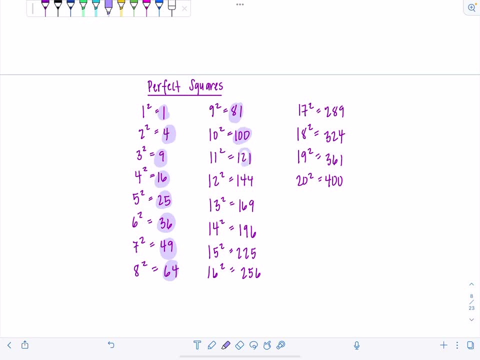 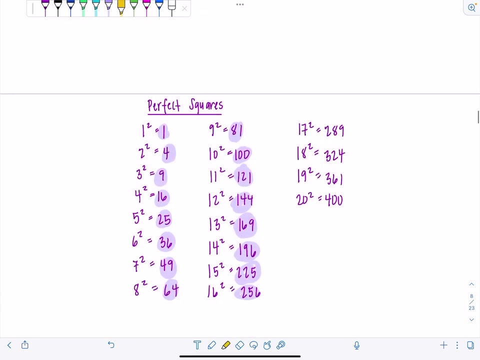 the largest perfect square that will divide evenly into the radicand that I can factor the radicand with okay. So here we're going to simplify: square root of 75.. Look at the purple ones that I've highlighted. What's the largest number from this list that divides evenly into 75?? 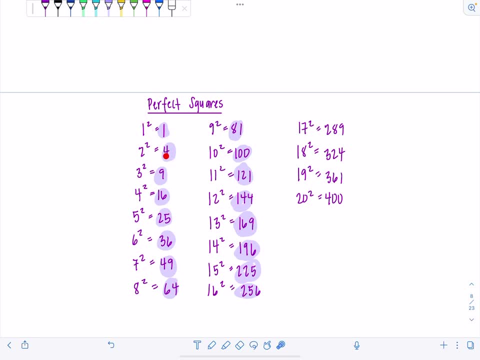 Okay, one is of no use, so just forget that guy. Four doesn't go into 75. Nine doesn't 16, doesn't 25 goes into 75. Ooh Shall, we keep going, just in case. Sure, Does 36 go into 75? No. Does 49? No? 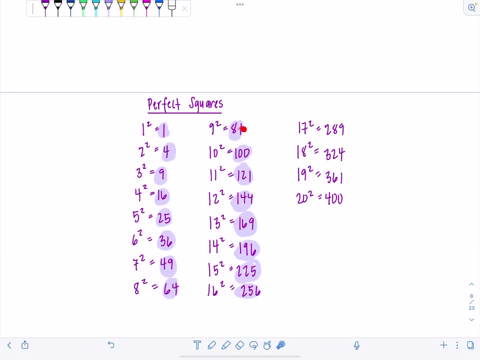 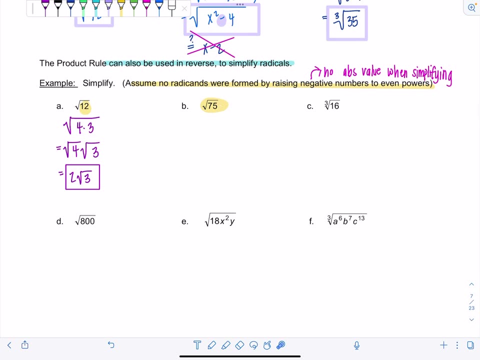 Does 64?? No, And now this is bigger than 75, so we don't need to keep checking. So 25 is the largest perfect square. So what you're going to do now is rewrite this as square root 25 times 3.. Good, Now break up the radical, so you're going to have square root of 25. 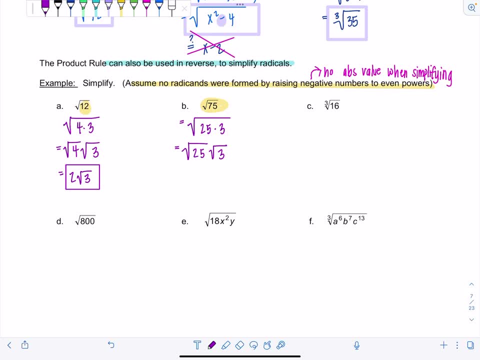 times square root of 3, and then square root of 25 simplifies to 5.. Okay, you would always write your answer with the constant that's not underneath the radical out front. You would not write it rad 3 and then the 5, because it's confusing. 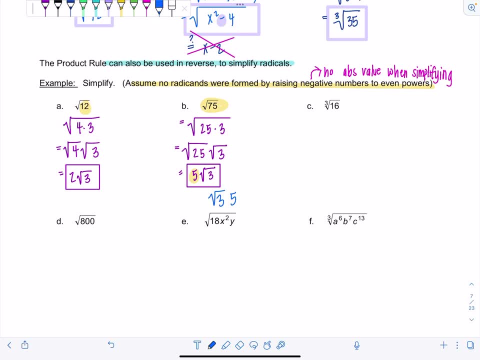 Is the 5 under the radical 2, and you just didn't draw the line long enough, You know. so we don't do that. We don't do it Okay. example C: We have the cube root of 16.. Yes, that means we need to know our perfect cubes as well. Mm-hmm, So perfect cubes. 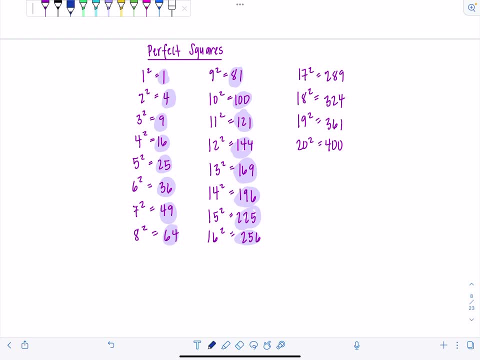 Let's make another list here. Perfect cubes, You don't need to know so many. They get big very quickly. Okay, obviously, one cubed is one 2 times 2 times 2, 8.. 3 cubed: 27.. 4 cubed: 64.. 5 cubed: 125.. 6 cubed- ooh, do you know? 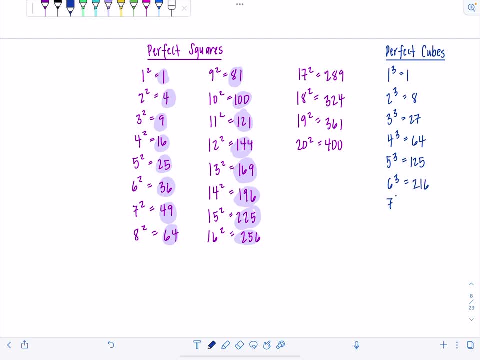 it 216.. Here's my favorite one: 7 cubed. Do you know why? 343.. I just think it looks so pretty. Look at that. 3 plus 4 is 7, as is you know this other 3 plus 4.. That's. 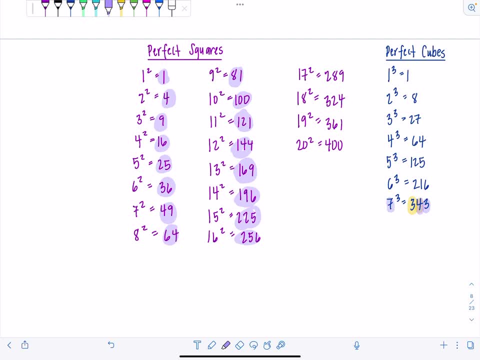 7 also, And then here's a 7. I don't know It just aesthetically looks fabulous to me, All right. Anyways, moving on, 8 cubed is 512, but I doubt you'll have to deal with. 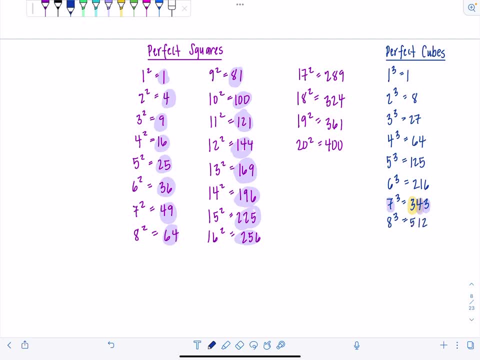 that Let's just go to 10.. 9 cubed- 729, and then 10 cubed. That's easy. That means it has three zeros. Okay, Now can you figure out what the largest number is from this list? Okay, That's going. 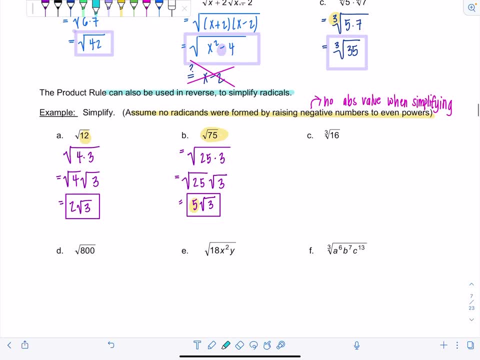 to divide evenly into 16.. Well, it's 8, right? You kind of can find them pretty quickly. So you're going to write this as cube root of 16 is 8 times 2.. Then split it up This: 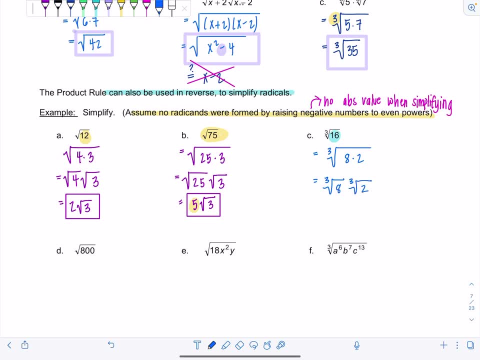 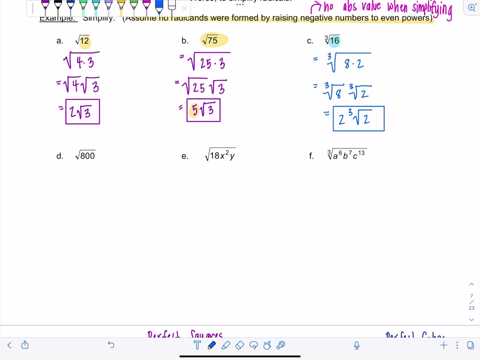 is cube root of 8 times cube root of 2.. So we're left with 2 cube root of 2.. Very good, Very, very good. Okay, Let's look at another example. Here we have square root of 800.. Okay, So take a second and think. 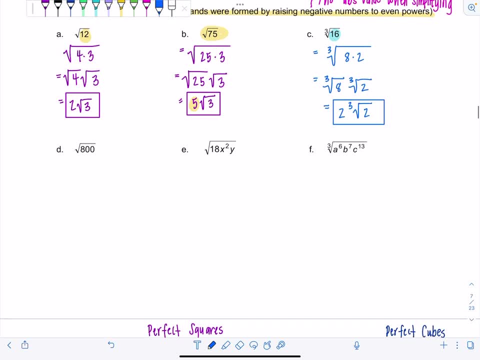 what's the largest perfect square that would go into 800?? Look at the list, See if you could figure out what the largest one is. So here, what must be going into 800? caught in the middle. So if I actually歩 100 times 2, it's already 800. 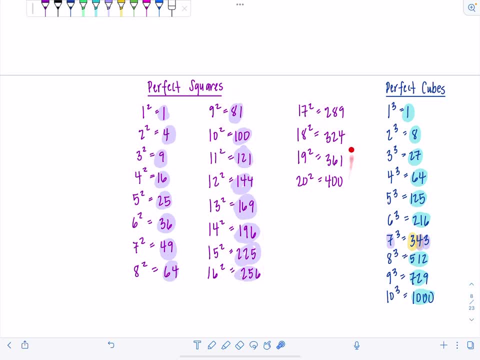 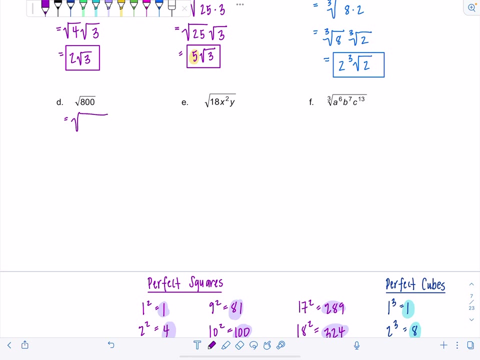 Imagine dividing the all of these numbers. that divides evenly into 800.. Can you spot it? It's actually four hundred, right? 400 times 2 is 800. So I can write this as square root: 400 times 2.. So that's square root of 400. Squared of 2, which is going to be 800. Right? Yes, Okay, Now try some numbers like this: Here we have square root of 0,ığını into docs. here it is always square root of 0, because we didn't add 2 and 3.. Okay, Here we are now. 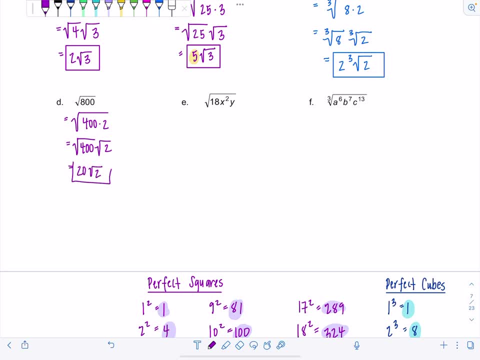 Where do we have square root of 2?? Where does 1 be? Here's square root of 1.. to be 20, rad 2.. Okay, Now, what if you didn't think of 400?? What if you saw a squared of 800? 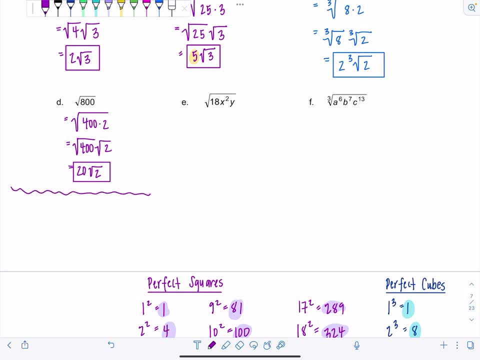 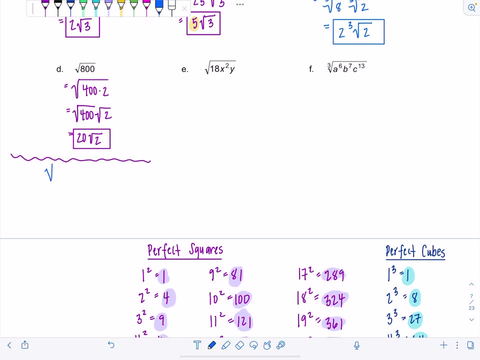 and, oh my, you got so excited, you just went for 100, right, You're like: oh, 100 is a perfect square, It goes into 800.. And you didn't even think to keep checking on the list. It's not the. 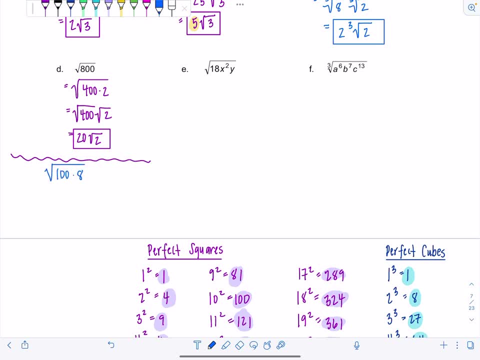 end of the world. Look what would happen. So you'd have 100 times 8, which you'd break up. So then that's square root of 100, square root of 8, which is 10 rad 8.. But then hopefully you would. 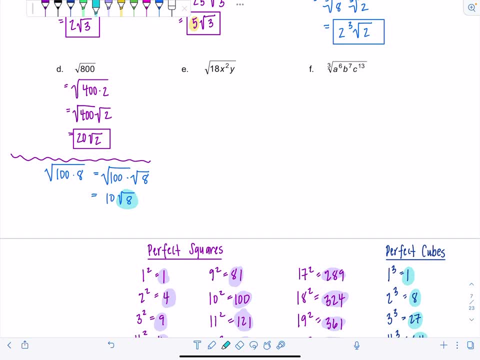 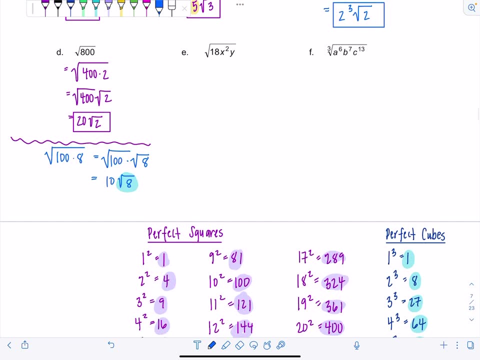 stop and take a look at things and think to yourself- wait a minute- that square root of 8 is not completely simplified. We just simplified square root of. well, we haven't simplified square root of 8 yet, So let's do it now. It would be 10 times rad. 8 is 4 times 2.. Yeah, So then it would. 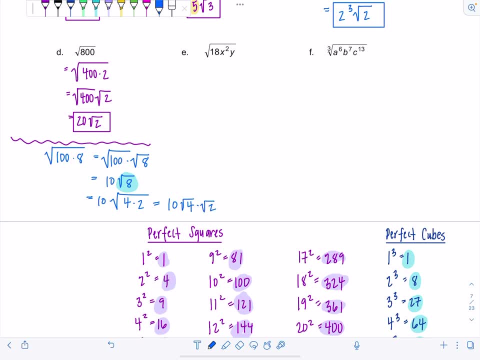 be 10 rad 4 times rad 2.. And then this rad 4, is 2.. So you'd have 10 times 2 rad 2,, which is 20 rad 2,, which is the same result. But look how. 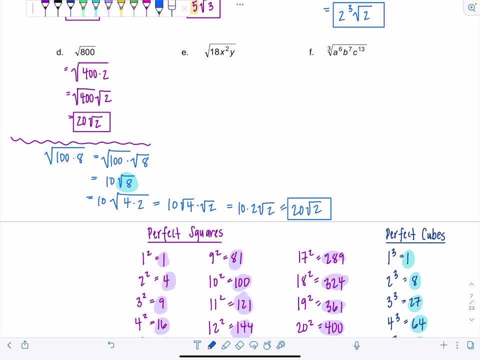 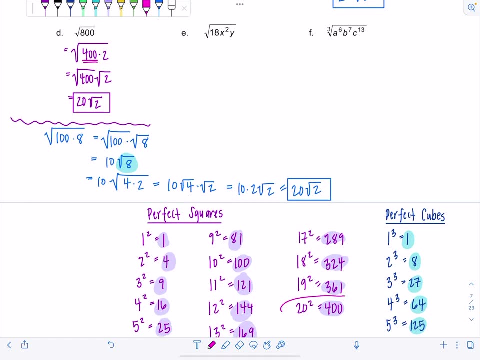 many more steps it took me. So always factor using the largest perfect square. okay, that you can divide evenly into the radicand. It will save you all this extra stuff. But you know, that's the beautiful thing about math, Even if you don't do it the most efficient way. 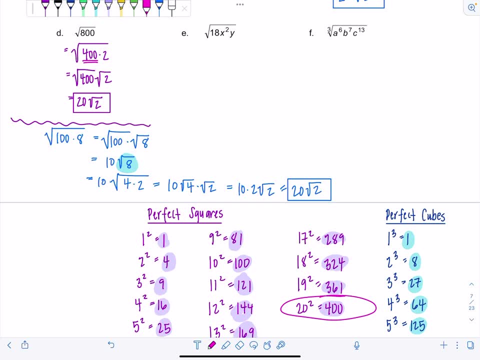 necessarily you can do it the most efficient way, So you can do it the most efficient way. But even if you don't do it the most efficient way, necessarily you can still get there by following the rules. You just might be the slow poke on the exam, You know, if you're one of those, 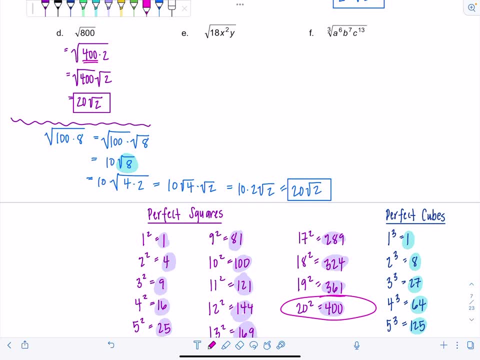 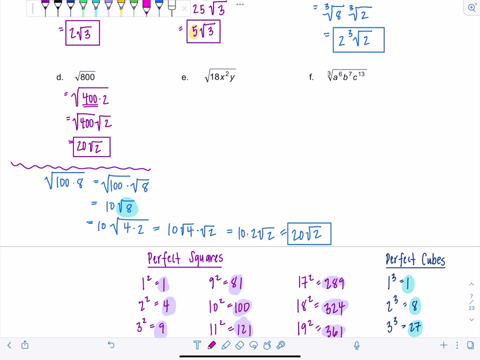 who's like I, always run out of time. maybe you're not doing things as efficiently as possible. Pay attention, Okay. Example E: Now we are getting fancy. We're involving variables with the constants. That's okay, We can handle it. So, square root of 18 x, squared y: I'm going to do. 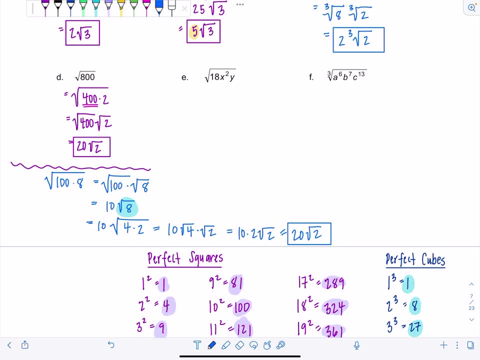 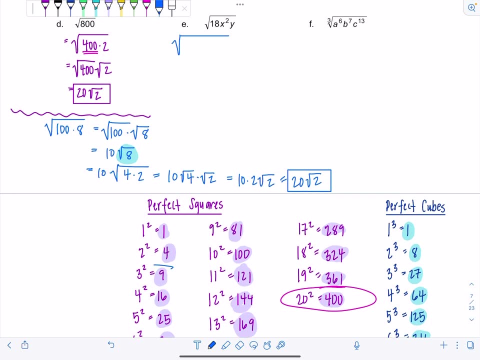 everything separate, 18.. How shall we break it up? What's the largest perfect square that goes into 18?? Can you see? It's just nine right, Because already 16 won't go in, and then 25 is too big. 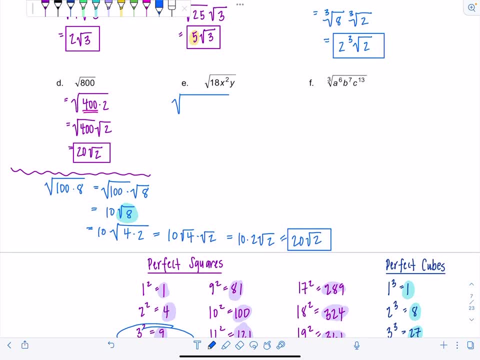 So this is going to be. let me do it like this. Let me do not such a big radical sign. I'll break up the number part separately. So we'll do square root of nine times two, And then I'm going to do square root of x squared and then square root of y, like this: Okay. 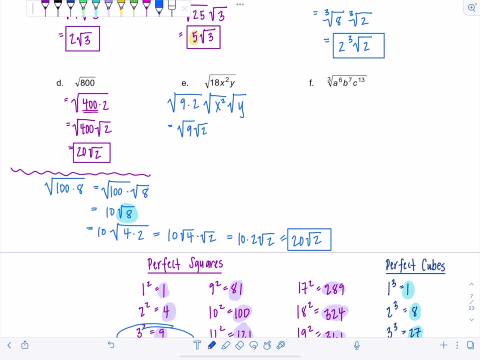 And then I'm going to split all the radicals up. So we have square root of nine, square root of two, square root of x, squared. square root of y, Square root of nine. that's three. Rad two stays rad two, Square root of x, squared. since they told me the variables aren't negative, I can just write: 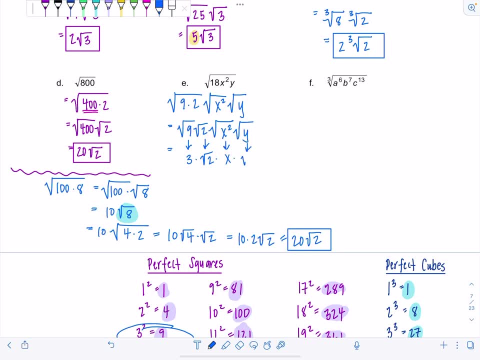 x, If they hadn't told me that I'd have to put absolute value x and then square root of y. just leave it as is. Okay. now everything's simplified. It just looks very ugly. So what we're going to do is everybody that's still trapped underneath the radical. they need to. 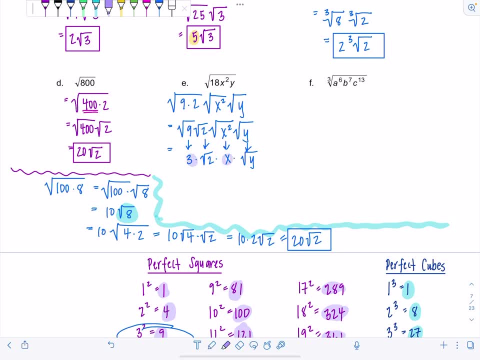 be together And then all the terms that are not underneath the radical go in the front of our final answer together. So you're going to have 3x rad and then put the two and the y together So they can keep each other company. you know They're trapped under that radical. 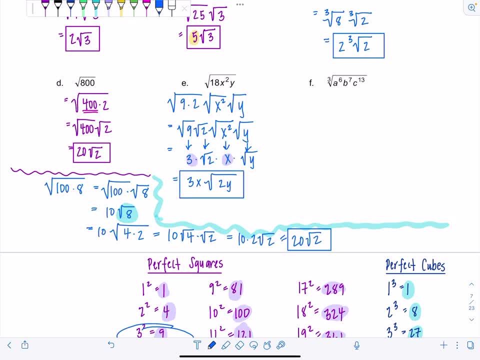 They don't want to be in solitude at the same time. All right, now for f. I'm going to show you a little bit of a diagram. So I'm going to show you a little bit of a diagram. So I'm going to. 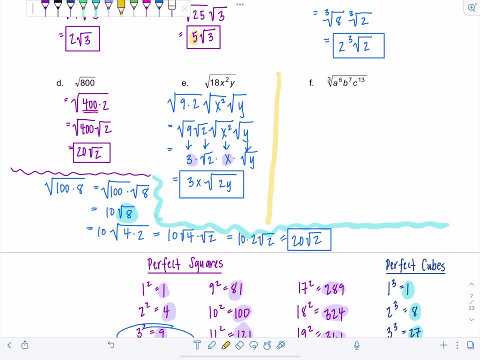 show you the longer way to do it, and then I'll teach you a little shortcut. Okay, you'll love it. Yes, Okay. so we'll split everybody up one at a time. So we have cube root of a to the sixth. 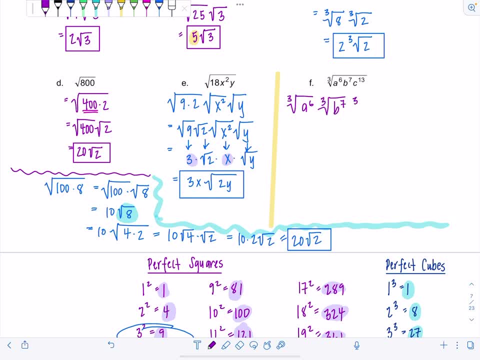 cube root of b to the seventh. cube root of c to the thirteenth. And how would you go about simplifying something like this? Well, a to the sixth. check what the index is. It's three, right. So how many a cubes can you write it as? You can write it as a cubed squared? 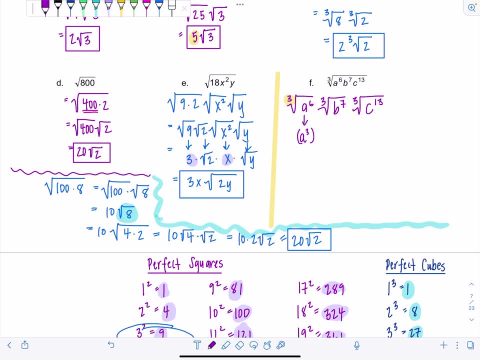 right, And then you take- or excuse me- a squared cubed other way around a squared, and I want it cubed That way. when I take the cube root it cancels. So then I'm just left with. 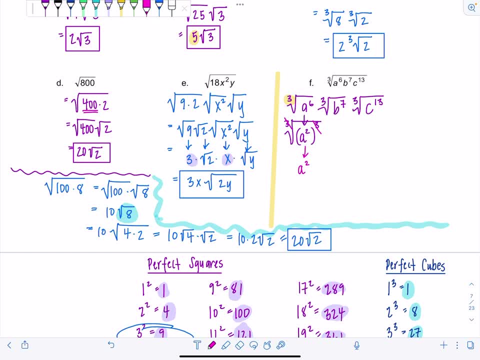 a squared. But an easier way of just doing that is you take the exponent on the variable and divide it by the index. Six divided by three gives me two, So just keep going with that, okay. Notice: here we have b to the seventh. Three does not divide evenly into seven. Three divides. 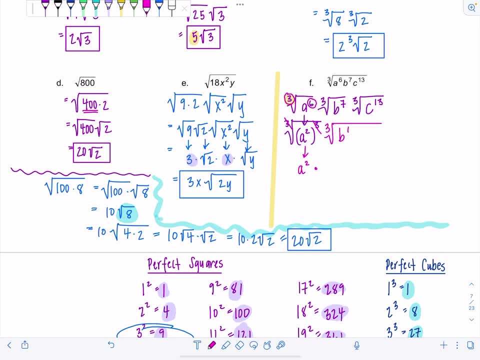 evenly into six, and then I have one more factor of b left over. So this would give me b squared, and then I still have cube root of b left over. Same thing here with this c to the thirteenth. Thirteen does not divide evenly by three. 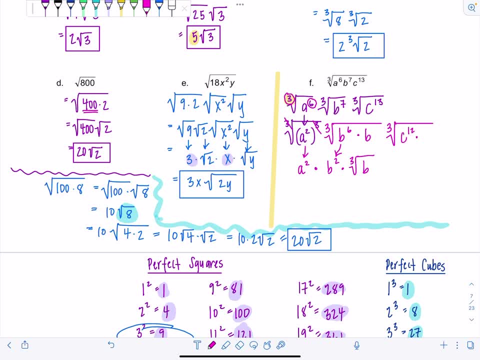 but twelve does Go for the largest number, that does. and then you still have another factor of c left over. Then twelve divided by three, this is going to be c to the fourth, and then cube root of c. okay, And then remember, everybody that's not underneath the radical is: 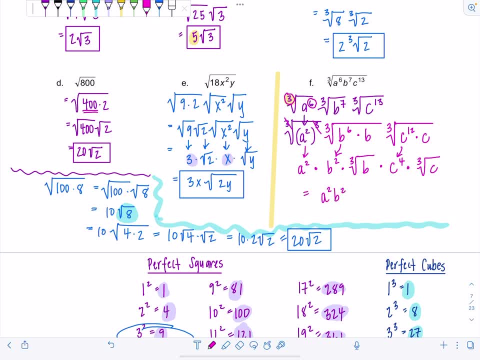 going to go out front together, So you're going to have a squared b, squared c to the fourth, and then cube root, who's still Trapped underneath. b and c, b and c. okay, Oops, So I told you I was going to show you a little. 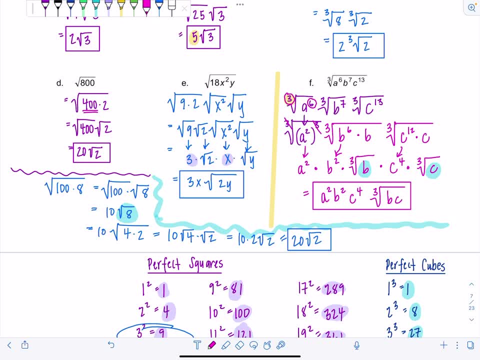 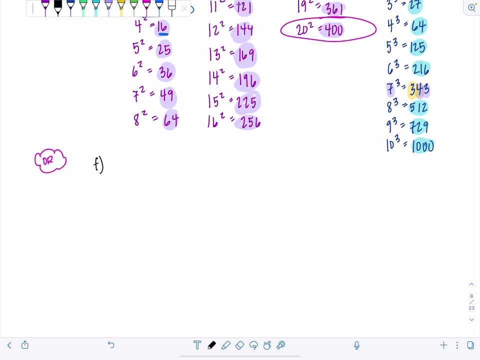 shortcut, right. So here's the idea: Save this method here, and then I'm going to rewrite this problem down below quickly, okay, Or you could have done it this way. So this is problem f. you have the cube root of a to the sixth, b to the seventh, c to the thirteenth. 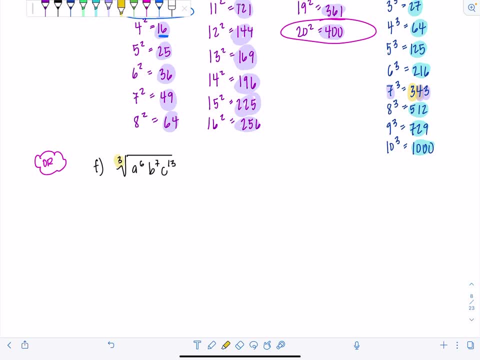 So you're just going to divide three into each of the exponents. Whatever the remainder is, it stays underneath the radical, okay, And the quotient comes outside. So six divided by three is two, right? Six divided by three is two, so I have a squared outside. 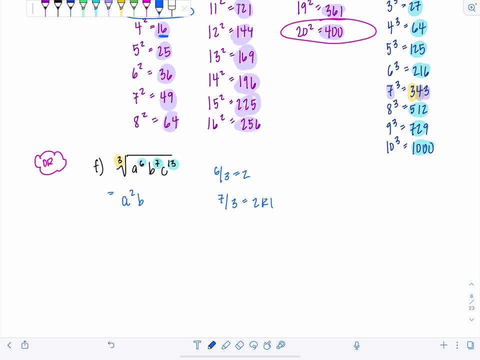 Six divided by three is two remainder one. So I have b squared. and then I have one b that's going to be trapped underneath the radical. Let me scoot this over. And then c to the thirteenth. So 13 divided by three, that's four remainder one. So that's why you have c to the fourth. 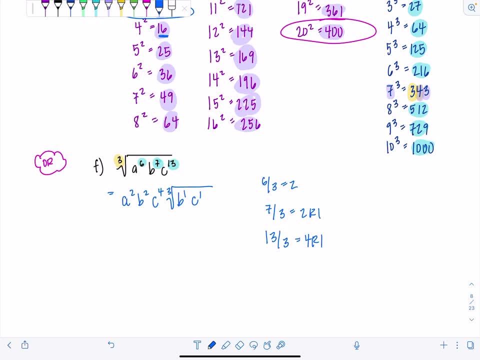 and then c to the first underneath, And then we know we don't have to put the one exponent. so that's how you just have a squared b squared c to the fourth cube root of b, c like that. Okay, so that's the quicker way. You could just do it without. 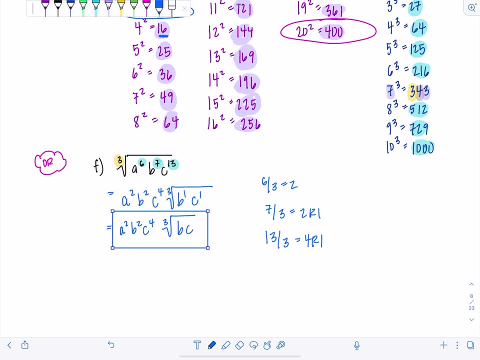 having to break up all the radicals, but do whatever feels comfortable for you so that you get the- you know the problem right And then, with practice, you might, you know, be able to do some of these steps in your head, like I'm showing you. Okay, a couple more g. 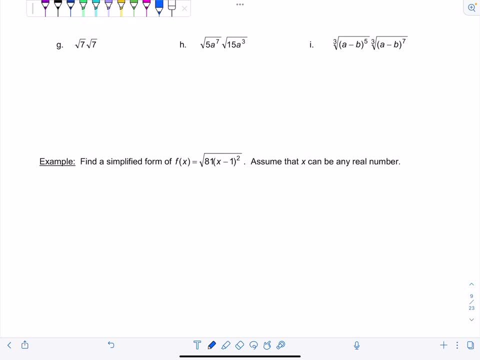 square root of seven times square root of seven. Okay so, square root of seven times square root of seven, That's going to be square root of 49, but then that just gives us back seven. Huh, Another way too that you could have thought of this is square root of seven times square root. 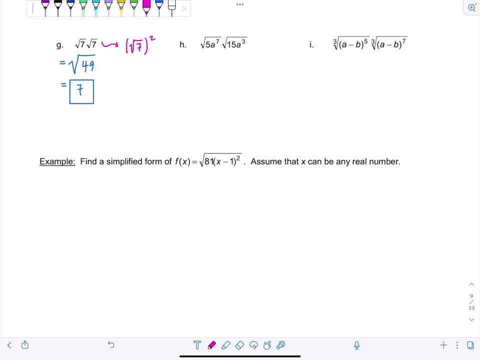 of seven means square root of seven squared. So if I square a square root, they cancel each other out and I just get seven. Oh, okay, very good. So keep that in mind. If you have square root of x times square root of x, it just gives you back x as long as. 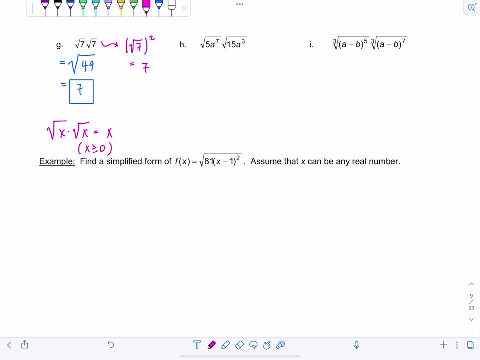 as you assume, x is greater than or equal to zero, And this is going to be very handy in a couple lessons in down the road. Okay, And we're going to rationalize denominators. Okay, h. square root of five, a to the seventh times the square root of 15, a cubed. 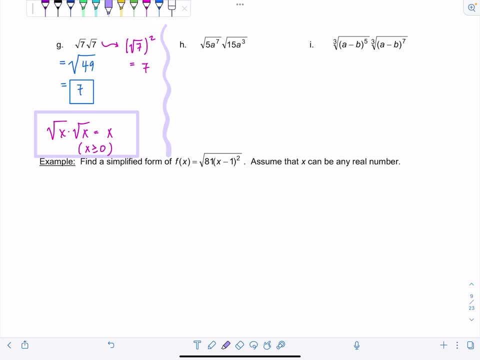 So you have a couple options. You could simplify each of the radicals as much as possible first, or you can multiply them and then just do it once at the end. That's usually what I prefer to do. So you have a couple options. You could simplify each of the radicals as much as possible. 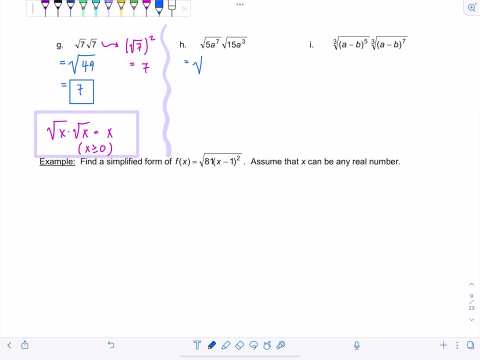 first, or you could simplify each of the radicals as much as possible. So I'm going to put one big radical, one big square root sign, and then multiply everything together. So I'll have five times 15,, that's 75, and then a. to the 10th right We add those exponents. 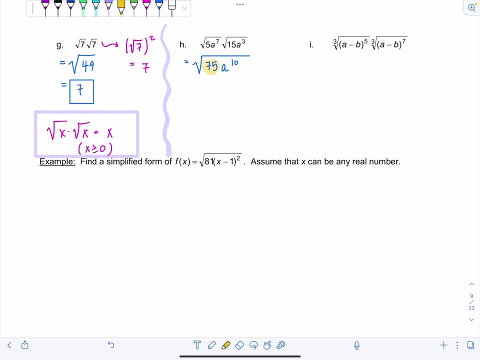 Okay, Square root of 75,. the largest perfect square that goes into 75 is 25.. So I'll write this as square root of 25 times three, and then we have square root of a to the 10th. Okay, Square root of 25, that's five. Square root of three stays Square root of a to the 10th. 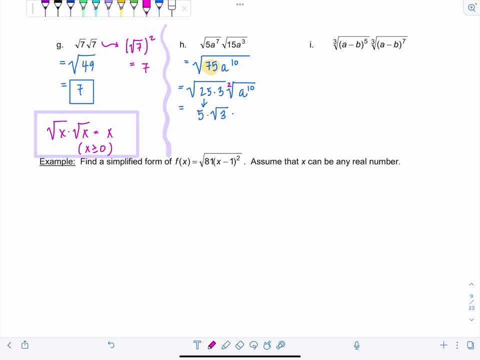 remember the index. right here is two that we're not writing, So this is going to be a to the fifth. Okay, Do we leave our answer like this? Certainly not. You're going to put five a to the fifth in the front and then you have square root of three like this. So lovely, Beautiful. 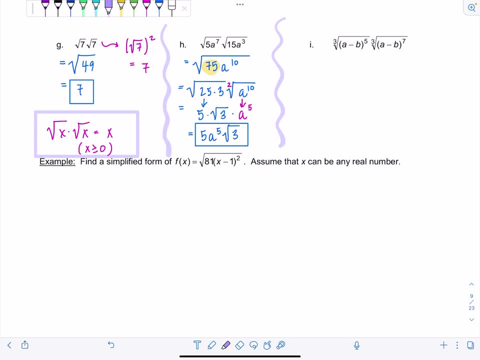 Okay, Last one here. Cube root of a minus b to the fifth times. cube root of a minus b to the seventh. So again I'm going to take a similar approach: Write one big radical and then I'm going to have a minus b, Remember. 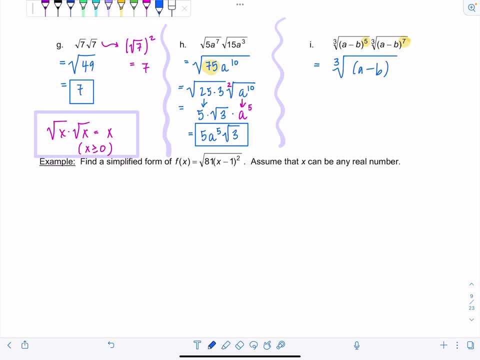 we're going to add these exponents. So five plus seven gives me 12.. And then how to simplify from here? we take this exponent and divide by the index. So 12 divided by three is four. So this is a minus b to the fourth. Okay, Very good, All right. Last example: here Find a simplified form of f of x. 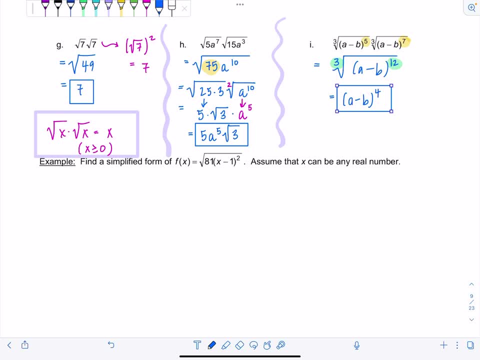 equals the square root of 81 times x minus one quantity squared. But watch out, Ooh. assume that x can be any real number. That means positive numbers, negative numbers, zero, No restrictions. So in simplifying this radical, I do have to be careful, since I'm taking 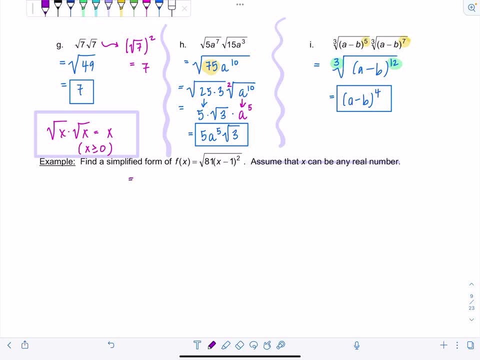 the square root of a variable quantity. Let's break it up. So f of x is going to equal square root of 81.. I'm doing it separately. Square root of x minus one squared square to 81, we know, is nine. And then, since x can be any real number, I have absolute value of x minus one, Remember. 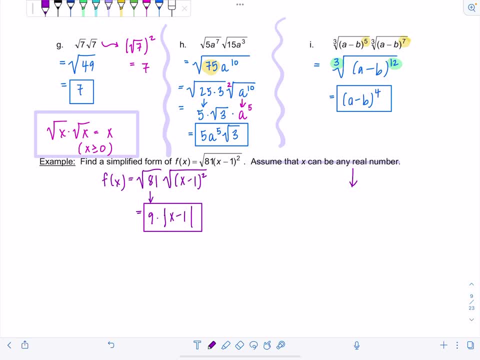 we covered this in the last lesson. So when x is any real number, generally speaking, the square root of x squared is equal to the exponent of degree. You can go any number you want. random equation General. you know you don't say anything about it, but do it all the way through same way again. 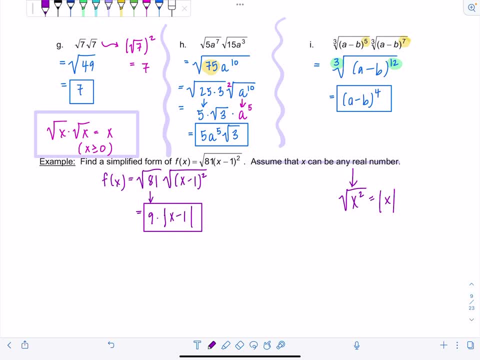 It's still a lot of work to do This long action that you did for me, So let's go into it. And then for a second, the absolute value of x. if you didn't catch the last video, i'll link it here, because i went into. 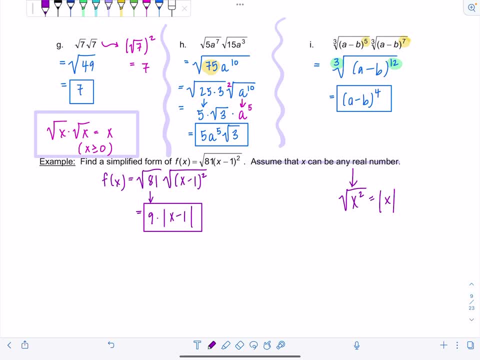 detail about why this is the case. okay, but it's very important and it will come up later in your math career. should you go on to study the beautiful subject that is calculus, you're going to have to be cautious about this, yes, okay, so best to learn it now with good habits, so you're not some sloppy. 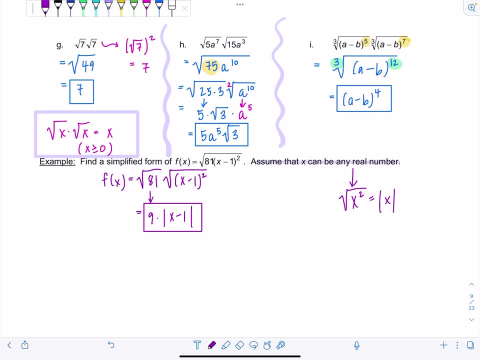 little mathematician running about having to undo some bad learned behavior later on. okay, that that concludes the lesson. hopefully it was short and sweet. and then next, you know, we did multiplying radicals. of course we're going to do dividing radical expressions and thank you so much for. 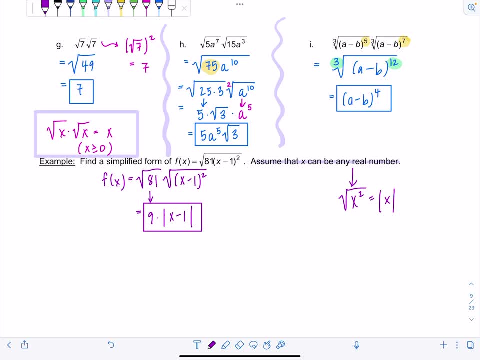 all your support. please subscribe and please hit that like button. give this video a thumbs up. hit the little notification bell. i noticed youtube has been unsubscribing some of you lovely people and i don't want that to happen. and then, if you're a more advanced student and you want some, 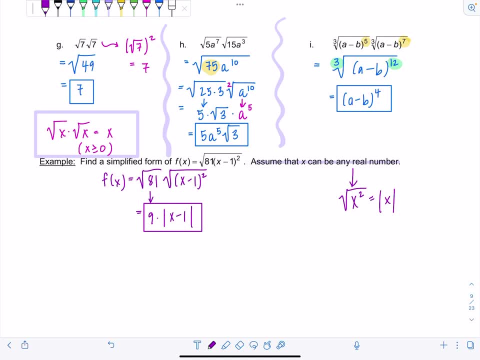 exclusive content access and sign up for my patreon. i'll link it here and hope everyone has a wonderful rest of their day. bye you.